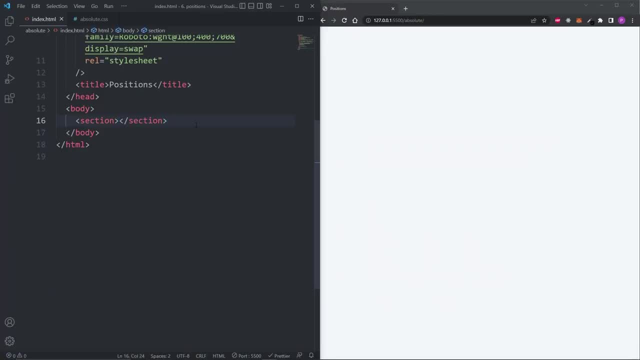 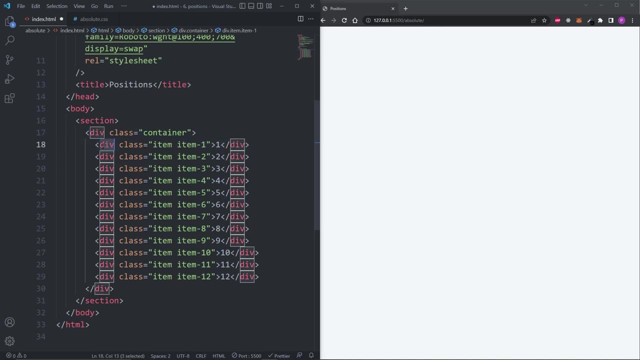 around. To start using CSS positions, we first need some elements in our HTML. All I have is a div with the class of container and 12 items nested inside of it. Each item is a div with the class of item and item 1,, 2,, 3 and so on. When I save, we see we actually have a grid. 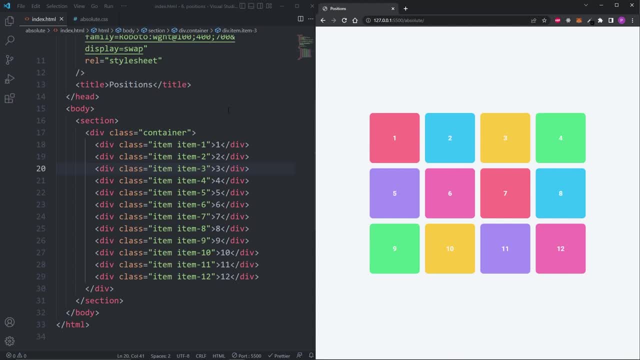 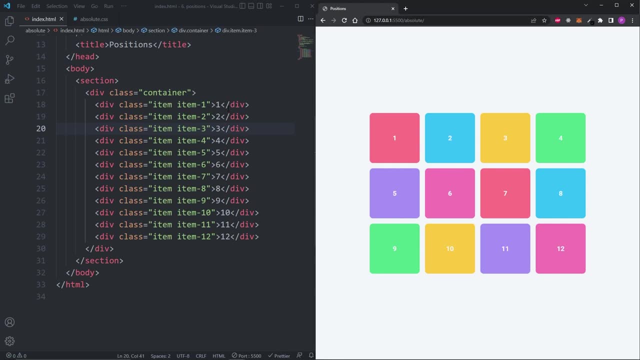 this is because I have some base tiles and a separate CSS file. None of this is relevant to CSS positioning. you don't need a container with 12 items and you don't need a grid to start using the CSS positioning properties. All of this is just for demonstration purposes. 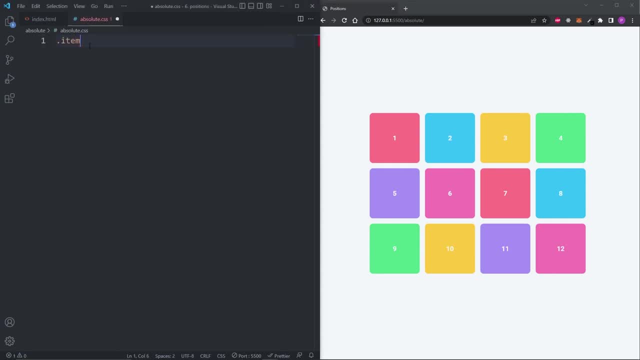 In a fresh CSS file I'll select the first item in our grid by its class name and give it the position property. In total, there are five position values: absolute, relative, fixed, sticky and static. When I set the position on our item 1 to absolute, we see that an item from 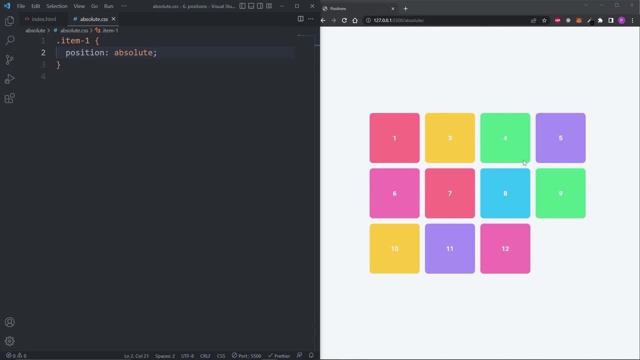 our grid disappeared. We have 1,, 3,, 4,, 5 and so on, but we don't see item 2, and this is because it's hidden underneath item 1.. To move item 1, we can use the top. 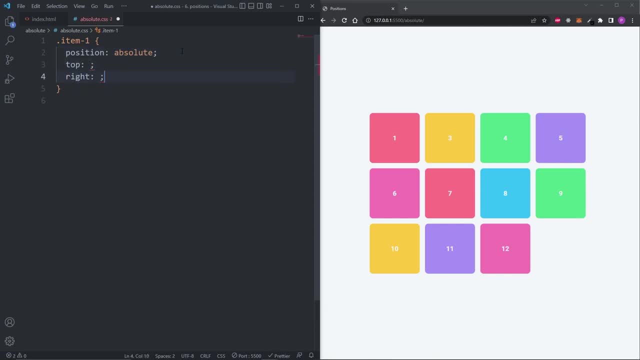 right, bottom and left properties. These properties are unlocked when we assign a position property to an element. If I give the top property the value of 0 pixels, we see now our item is positioned at the top of the page And also the reason we're missing an item from. 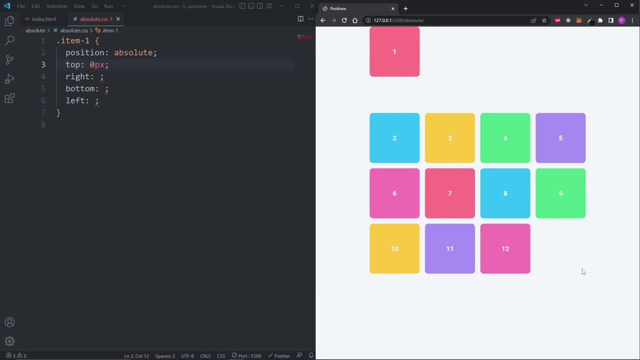 our grid is because when we set item 1 to have a position of absolute, item 1 got removed from the grid. Actually, it got removed from the entire document. Elements that are assigned a position of absolute are removed from the document. No space is created for them and other. 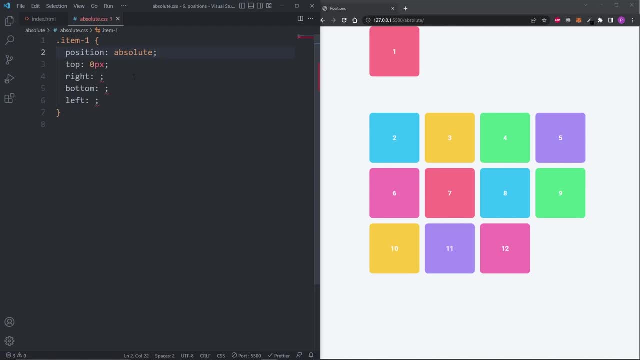 elements will behave as if that element never existed. If I set left to 0 pixels, now our item is on the top left corner. If I set the bottom to 0 pixels, nothing happens. This is because it doesn't make sense to have both a top and a bottom. I can comment out the top property and now with: 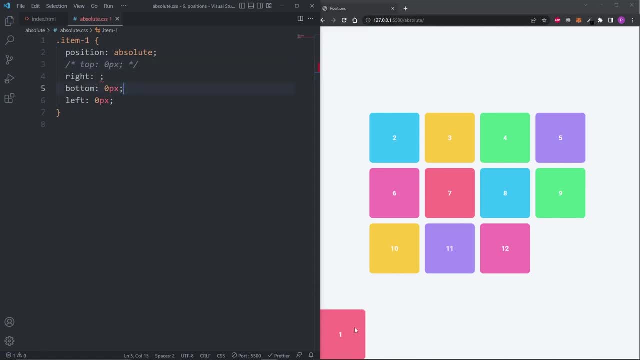 the bottom of 0 pixels, we see that the element is positioned at the bottom left corner. The same goes for the left and right properties. I use one of them, but not both at the same time. I'll comment out the left property and set the right property to 0 pixels. I'll also comment. 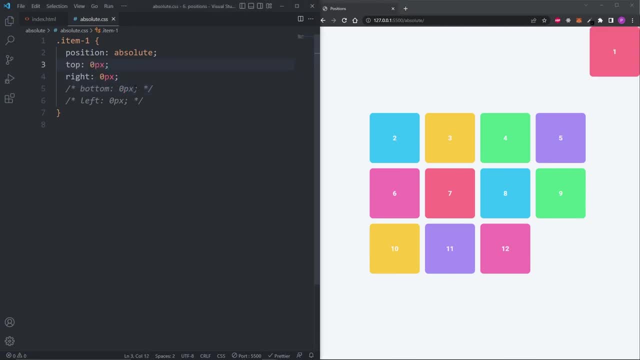 out the bottom property and set the top property to 0 pixels. Now our item is positioned at the top right corner. but what happens if I give our top and right properties some negative numbers? I'll set both to minus 50 pixels and now our item is half visible. This is pretty cool. 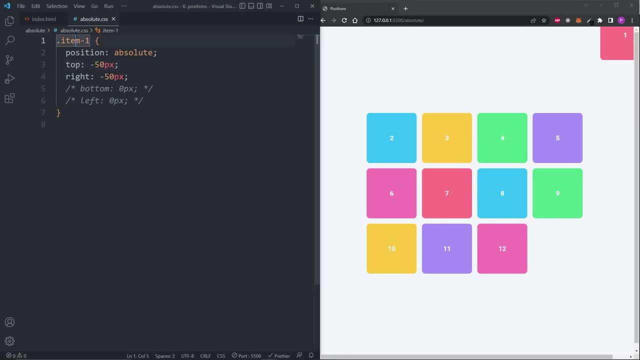 but we've got some horizontal scrolling. I can select the body and give it the overflow x of hidden, And now the horizontal scrolling is gone. Did you notice, whenever we were defining values on the top, right, bottom and left properties, that those values were positioning? 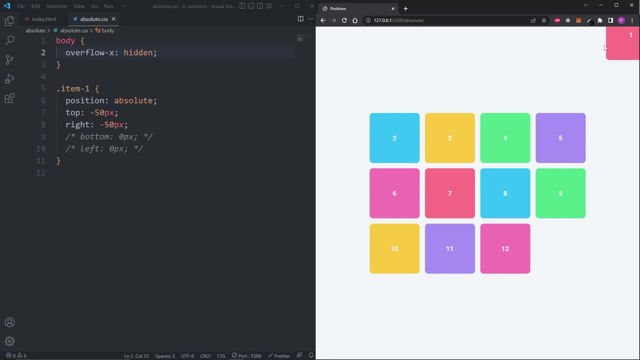 item 1 relative to the entire page Minus 50 pixels on the top and right properties places item 1 at the top right corner of the entire page. If I wanted item 1 to position itself relative to its parent, then we need to select the parent and give it a position. 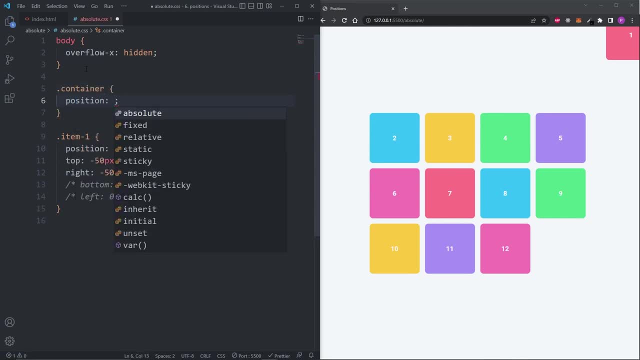 Any position value will work except static. because static is the default value, I'll set the position to relative, and now we see item 1 is being positioned relative to the parent instead of the entire page. The way this works is over on the HTML. 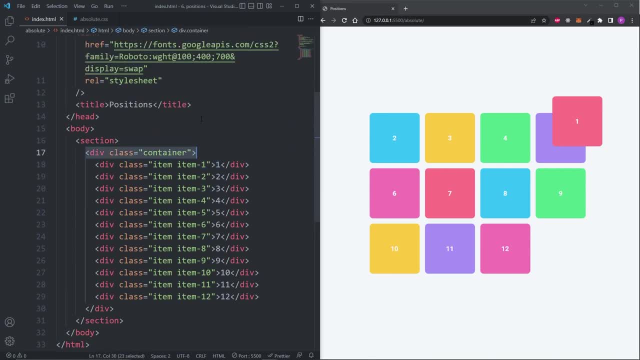 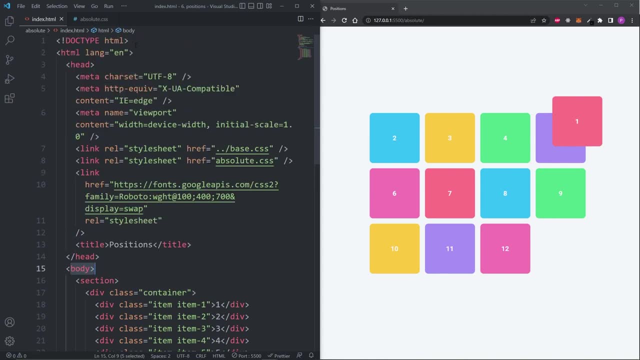 item 1 is asking the parent whether it has a position property. If not, then it asks the next parent, and then next, and then next, until it finds one with a position property defined, And if it doesn't find one, then it defaults to being positioned relative to the HTML element. 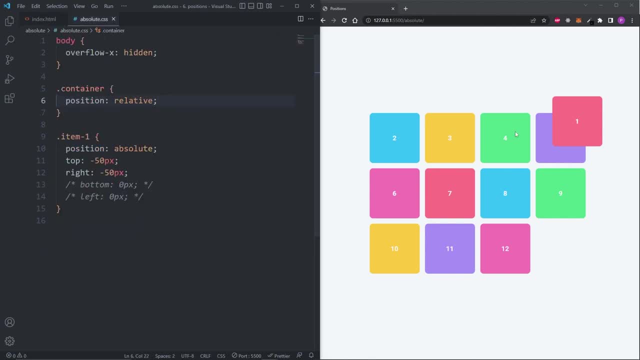 Now that item 1 is being positioned relative to the container, it's stacking itself above item 5.. If we wanted item 1 to be layered underneath item 5, what we can do is use the z-index property and set it to minus 1.. 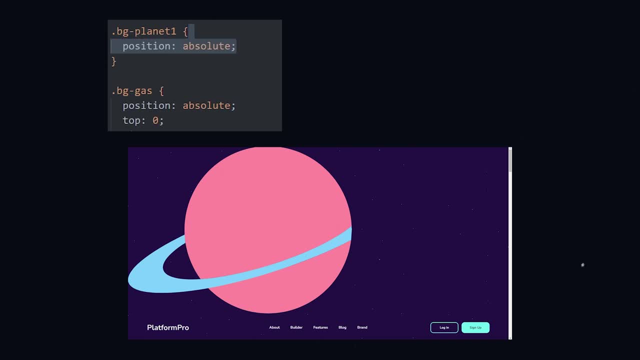 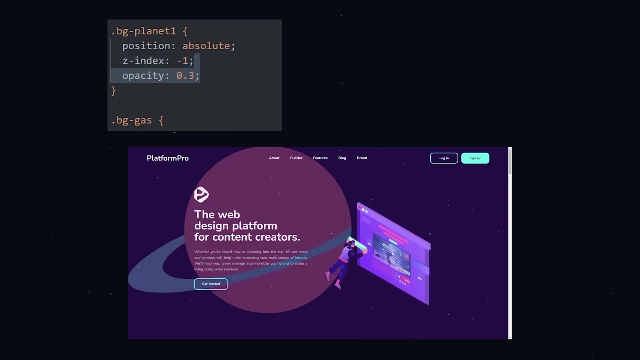 Back on my client's website. I give the planet the position of absolute. The planet is now removed from the document but is stacking above other elements. I use the z-index property to layer the planet underneath the other elements. Also, I give the planet an opacity of 0.3, because the planet is way too bright. 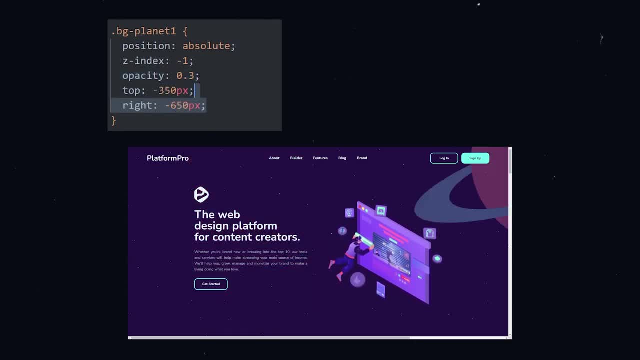 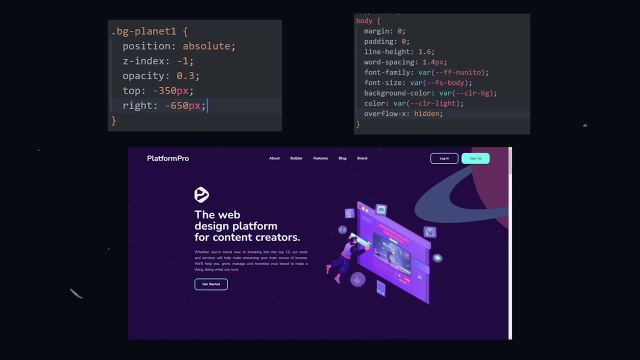 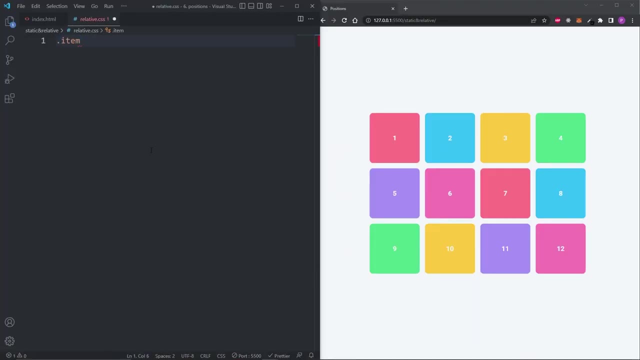 I played around with the top and right properties until I was happy with the position and I also added an overflow x of hidden on the body to remove the horizontal scrollbar. And finally, I repeated the same process for all the other images. If I select item 1 and give it the position of static, we see nothing happens. 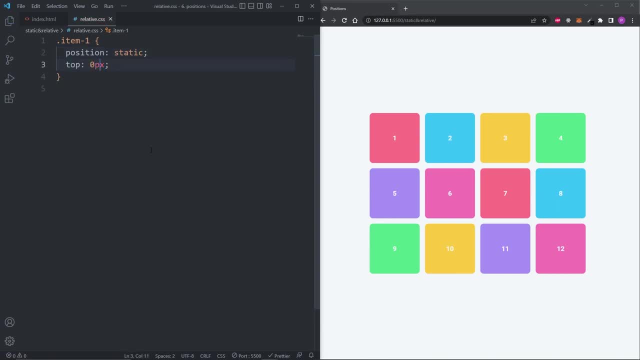 If I give it a top property of 0 pixels, nothing happens. If I set it to 1000 pixels, still nothing happens. Nothing is happening because static elements don't have access to the top, right, bottom and left properties, nor do they have access to the z-index property. 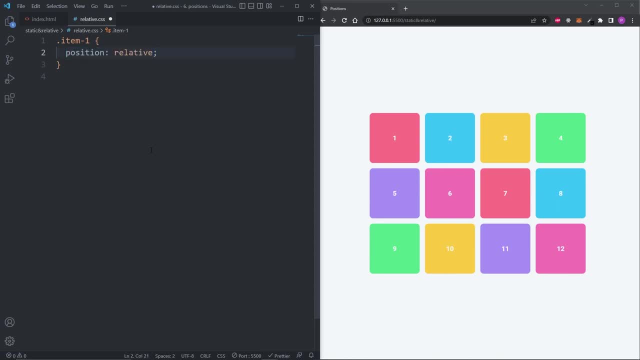 Instead of that, I give it a position of relative. We see nothing happens. but unlike it, relative has access to the top, right, bottom, left and z-index properties. If I give it a top property of 0 pixels, it doesn't move. However. 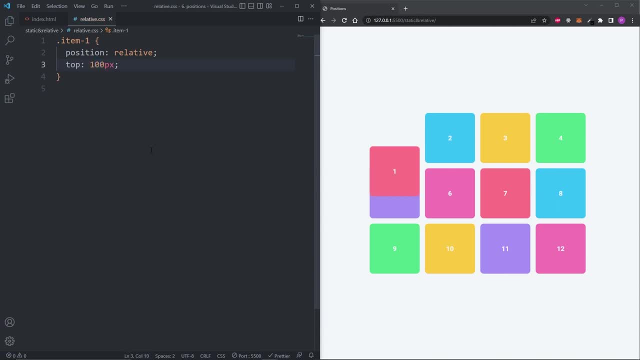 if I set it to 100 pixels, we see it pushed it 100 pixels away from the top. If I give it a top property of 100 pixels, we see it pushed it 100 pixels away from the left, Unlike the position of absolute elements with the px. there are no options. Take action. 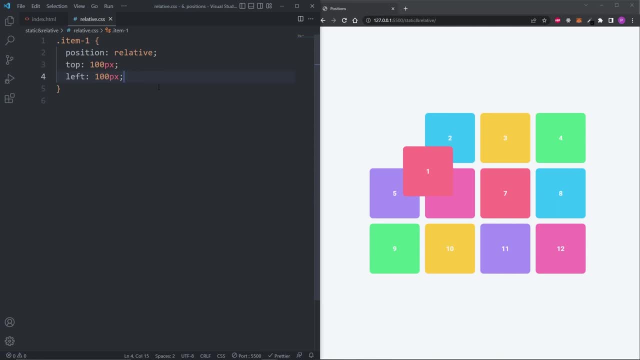 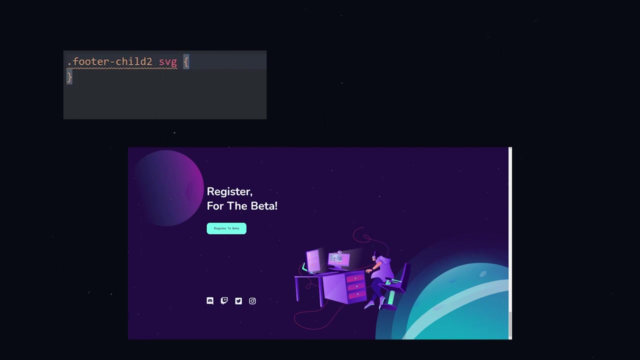 elements with the position of relative remain in the normal flow of the document. Use relative when you want to keep your element in the normal flow of the document and use absolute when you want to remove your element from the normal flow of the document. On the footer, I want to push this animation slightly towards the right. normally I would 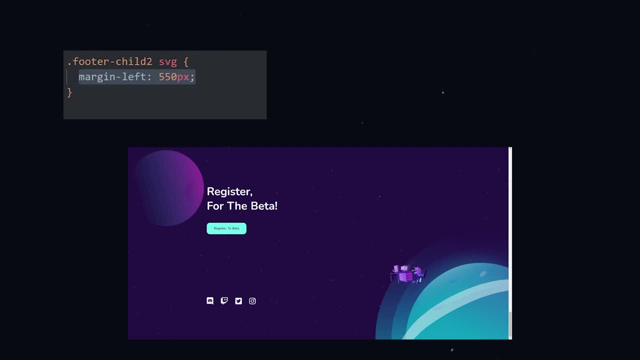 just use a margin left. but in this case I can't, because I set the width and height with percentages and if I use margins the animation would shrink. So what I can do is give the animation the position of relative and use the left property. 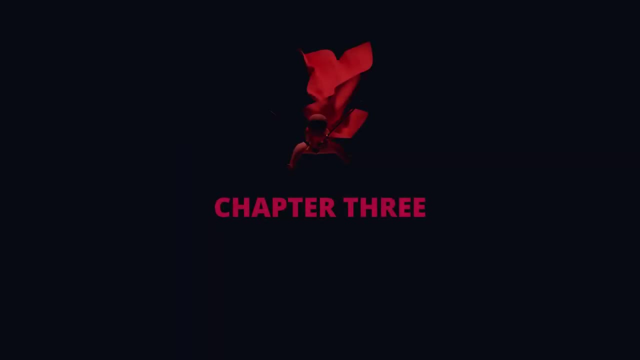 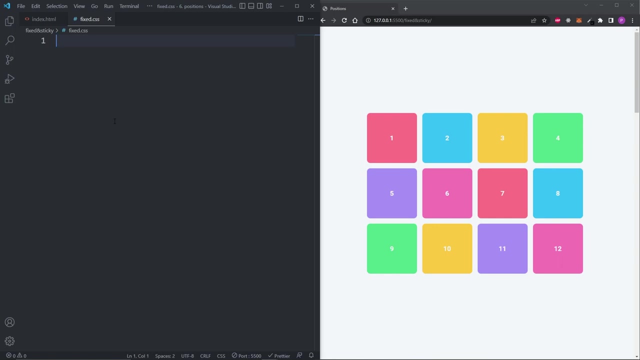 to push it slightly to the right without it shrinking. The two final positions are fixed and sticky. they both stick an element into position but they do it slightly differently. Fixed actually behaves very similarly to the absolute position. Like absolute, elements with the position of fixed are removed from the document. 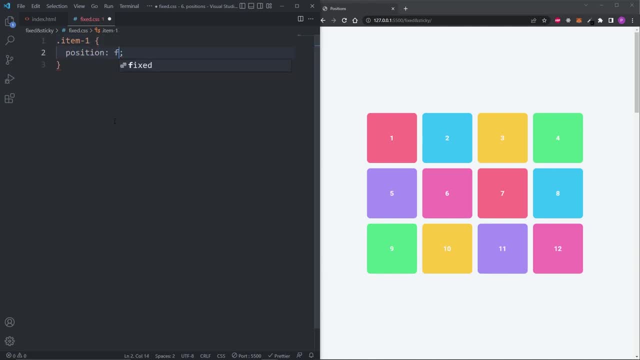 So when I set item 1.. 1 to a position of fixed, we get the same behavior as we did when we were working with absolutes. item 1 was removed from the entire document and is currently layered on top of item 2, which is why we don't see item 2.. 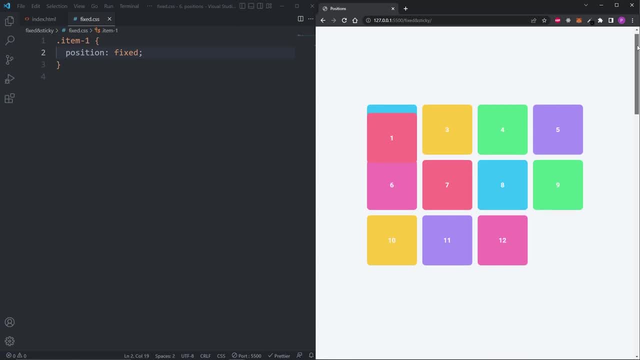 However, one area where fixed is different than absolute is when we start scrolling, We see item 1 is now following us when we're scrolling the page. The second area where fixed differs from absolute is: unlike the absolute element, a fixed element is always positioned relative to the HTML element.